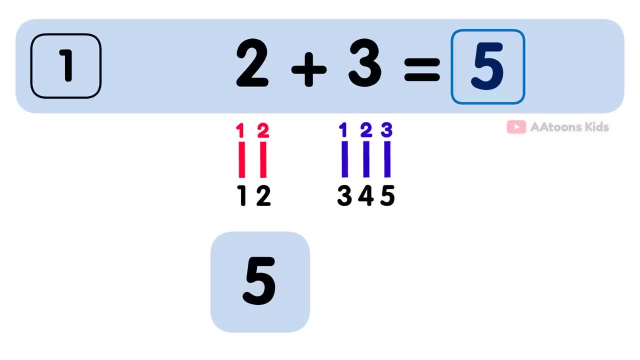 to 2 plus 3 is 5.. 4 plus 5 is equal to 9.. Let's add the numbers 4 and 5.. 4, 5.. Now count together 1,, 2,, 3,, 4, 5.. So the answer: 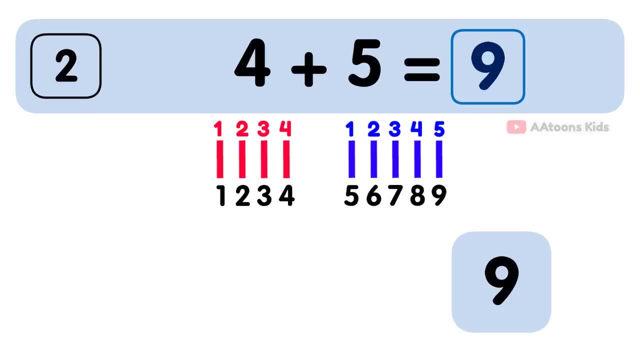 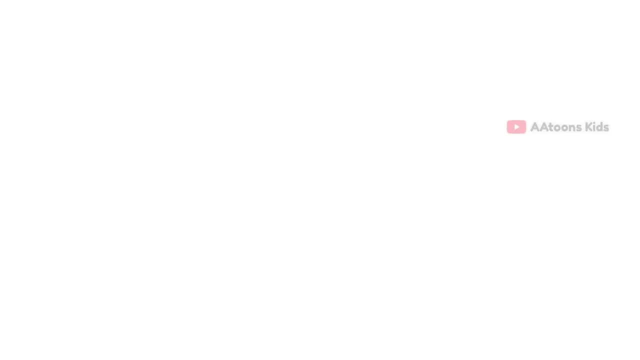 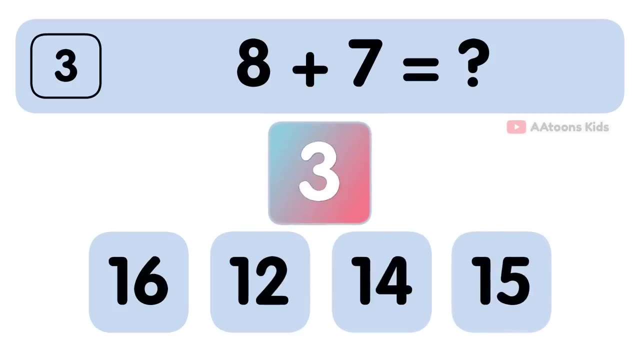 to 4 plus 5 is 9.. 5,, 6,, 7,, 8,, 9.. So the answer to 4 plus 5 is 9.. 8 plus 7 is equal to 15.. Let's add the numbers 8 and 7.. 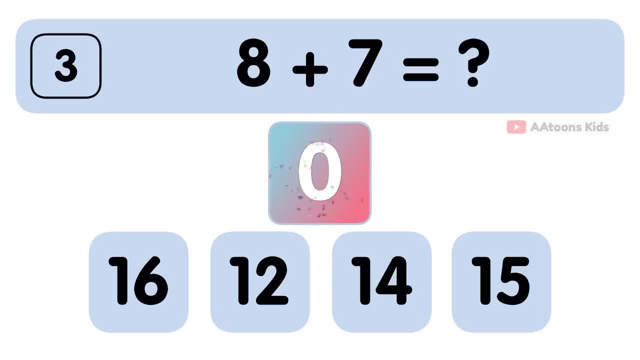 6 plus 7 is 8.. 6 plus 7 is 9.. 8 plus 7 is equal to 7. 15. Let's add the numbers 8 and 7. 8 and 7 is equal to 8.. 2 plus 8 is equal to 13.. 8 plus 7 is going to become 15.. The same goes for the third fraction sorted to 1 plus 3.. 9 plus 2 is going to become 17.. And 2 from the number from 3 to 13 becomes 18.. 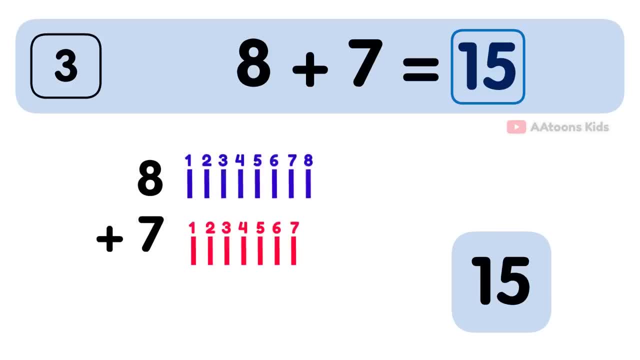 8 and 7 increase to 3.. Now count down the numbers 8, 7.. Now count together 1,, 2,, 3,, 4,, 5,, 6,, 7,, 8,, 9,, 10,, 11,, 12,, 13,, 14,, 15.. So the answer. 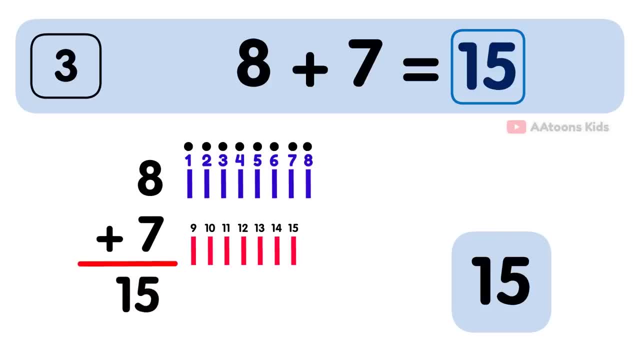 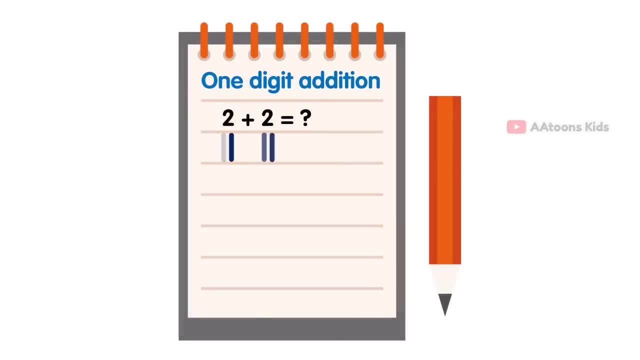 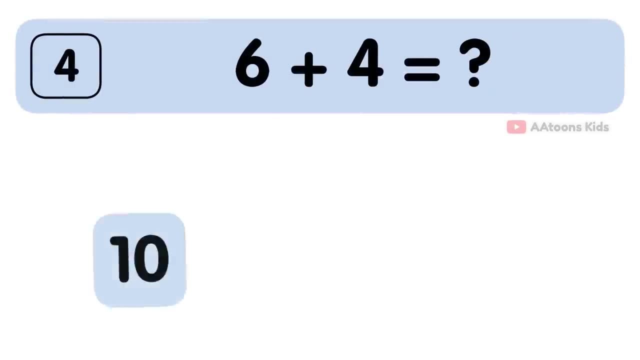 to 8 plus 7 is 15.. Now open your notebook and pencil and do yourself To attempt the quiz. click on the link in the description. 6 plus 4 is equal to 10.. So the answer to 6 plus 4 is 10.. 1 plus 9 is equal to. 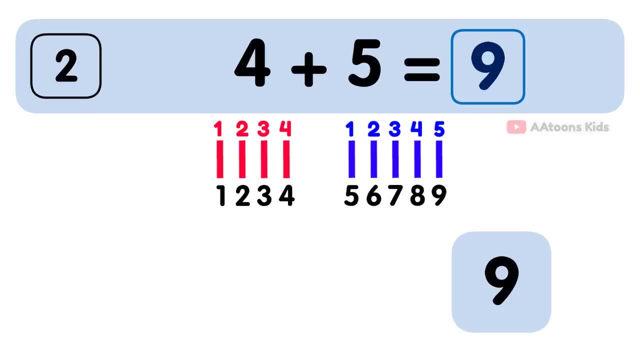 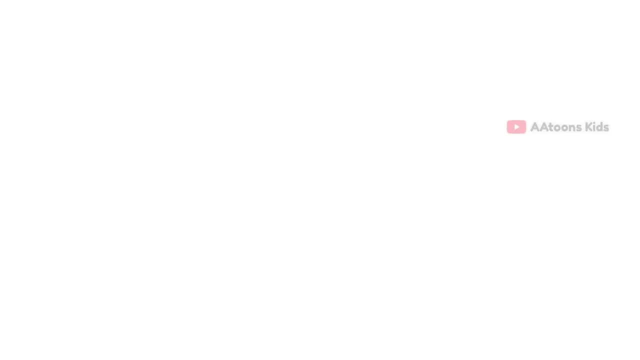 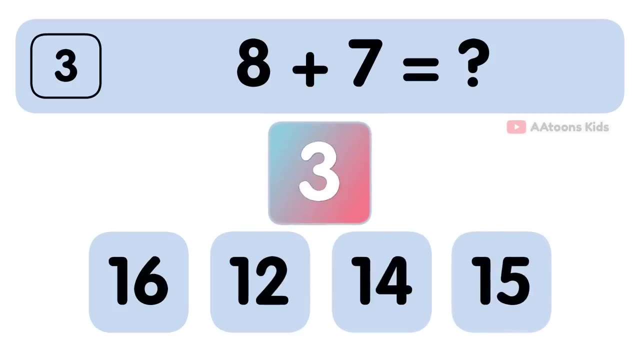 to 4 plus 5 is 5.. 6,, 7,, 8,, 9.. So the answer to 4 plus 5 is 9.. 8 plus 7 is equal to 15.. Let's add the numbers 8 and 7.. 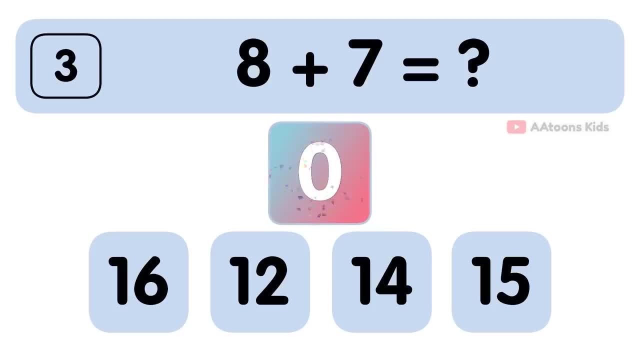 2 plus 7 is equal to 9.. So the answer to 2 plus 5 is 3.. 4. Let's add the numbers 6 and 6.. 9.. Now count together 1,, 2,, 3,, 4, 5. So the answer to 4 plus 5 is 9.. 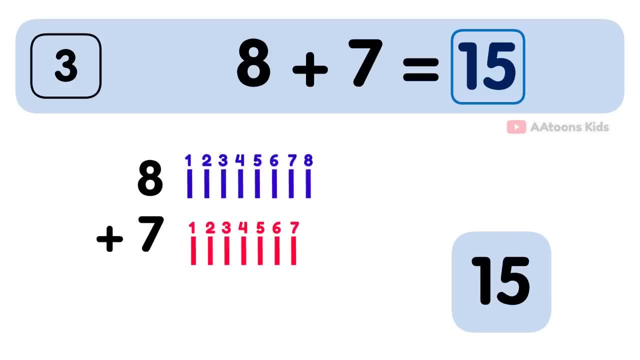 8, 7.. Now count together: 1,, 2,, 3,, 4,, 5,, 6,, 7,, 8,, 9,, 10,, 11,, 12,, 13,, 14,, 15.. So the answer: 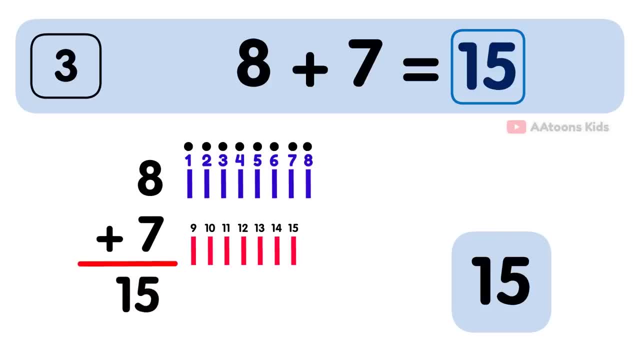 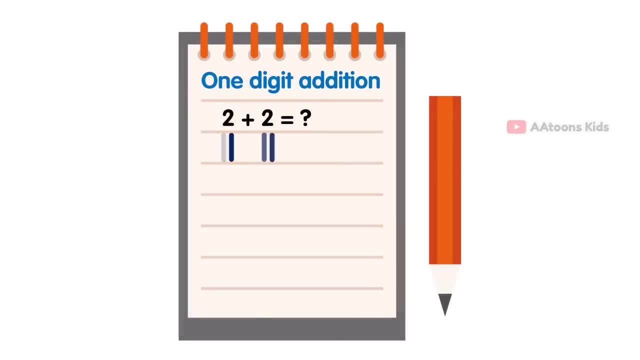 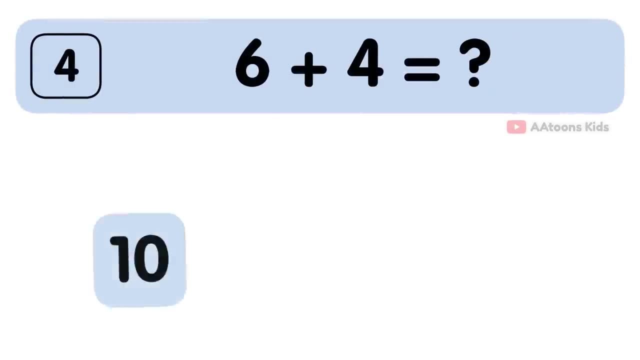 to 8 plus 7 is 15.. Now open your notebook and pencil and do yourself To attempt the quiz. click on the link in the description. 6 plus 4 is equal to 10.. So the answer to 6 plus 4 is 10.. 1 plus 9 is equal to. 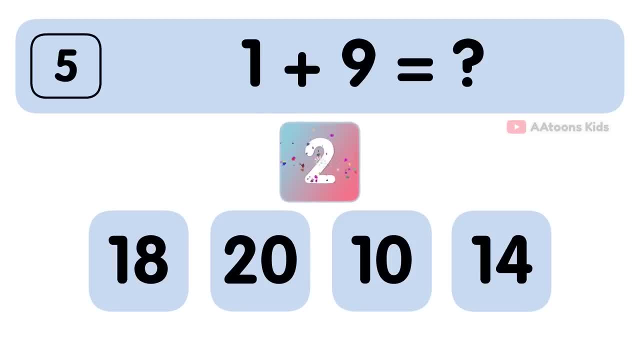 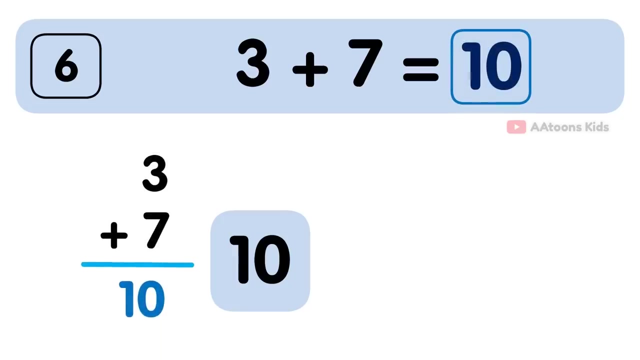 10. So the answer to 1 plus 9 is 10.. 3 plus 7 is equal to 10.. So the answer to 3 plus 7 is 10.. 5 plus 2 is equal to 10.. So the answer to 5 plus 2 is equal to. 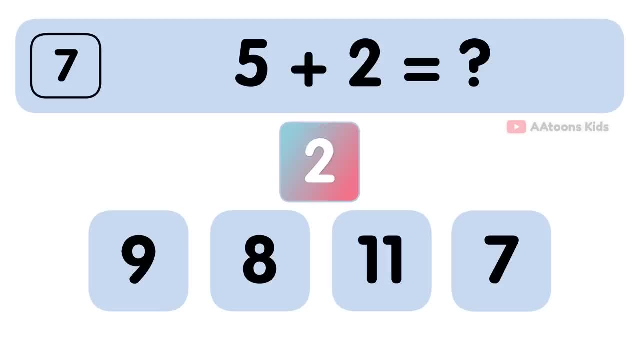 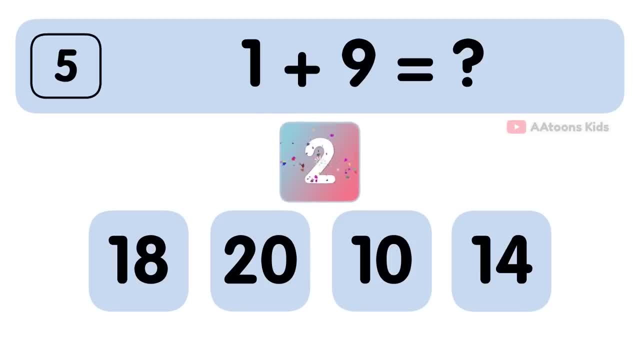 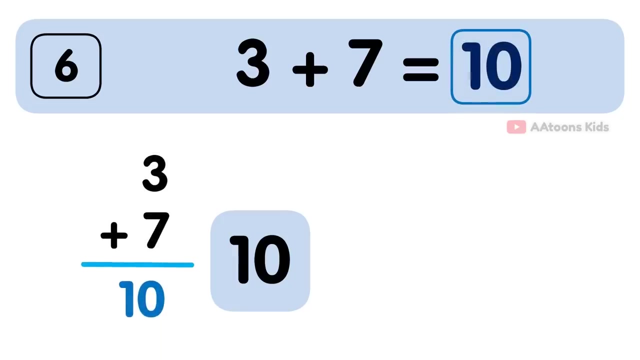 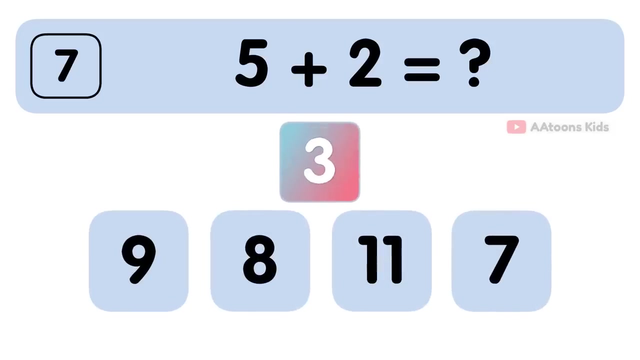 10. So the answer to 1 plus 9 is 10.. 3 plus 7 is equal to 10.. So the answer to 3 plus 7 is 10.. 5 plus 2 is equal to 10.. 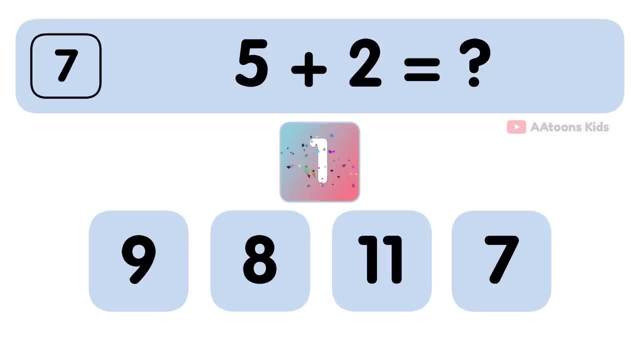 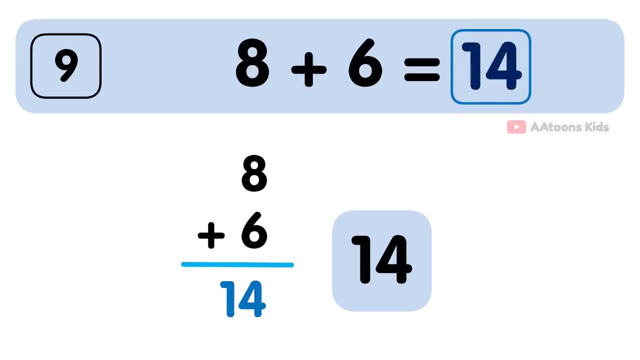 7. So the answer to 5 plus 2 is 7. 3 plus 3 is equal to 6, So the answer to 3 plus 3 is 6. 8 plus 6 is equal to 1, 2, 3, 14.. So the answer to 8 plus 6 is 14.. 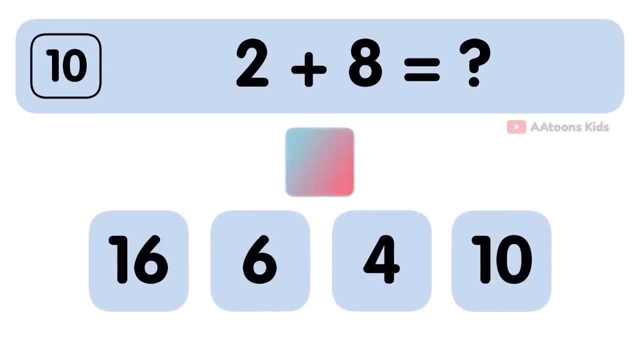 2 plus 8 is equal to 10.. The answer to 2 plus 8 is 10.. 3 plus 4 is equal to 7.. The answer to 3 plus 4 is 7.. 6 plus 5 is equal to. 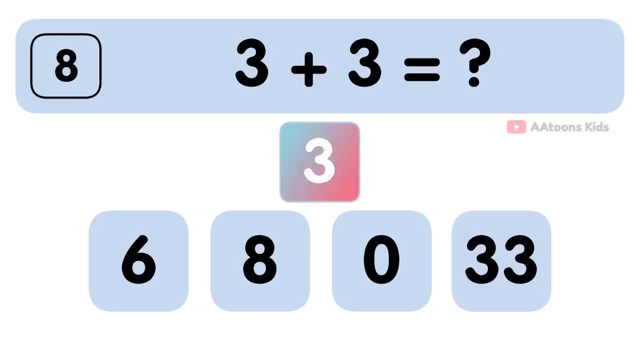 6. So the answer to 3 plus 3 is 6. 8 plus 6 is equal to 6. 8 plus 6 is equal to 14.. So the answer to 8 plus 6 is 14.. 2 plus 8 is equal to. 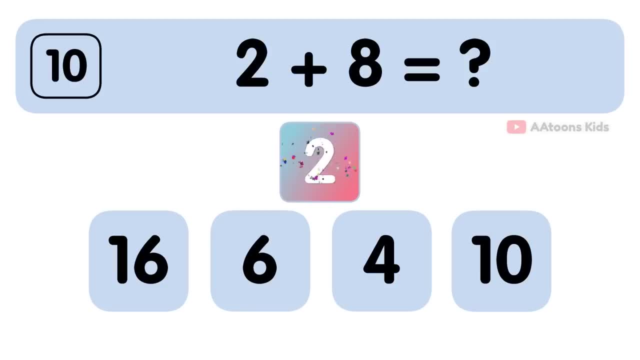 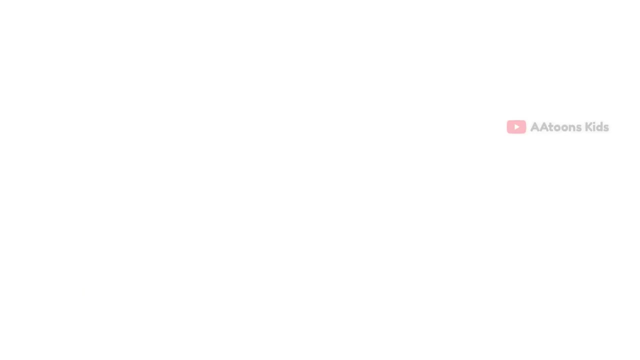 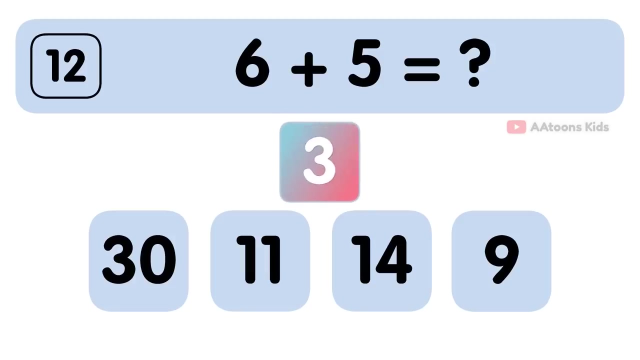 10.. The answer to 2 plus 8 is 10.. 3 plus 4 is equal to 7.. The answer to 3 plus 4 is 7.. 6 plus 5 is equal to 11.. The answer to 6 plus 5 is 11.. 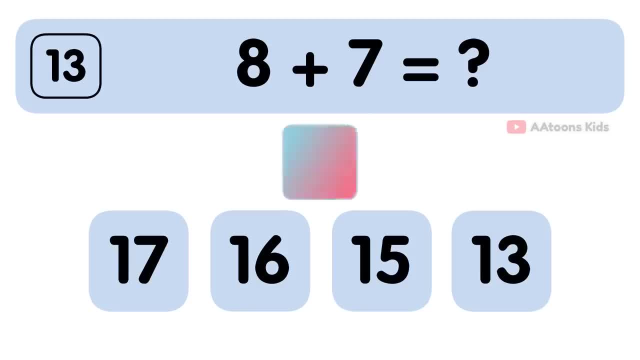 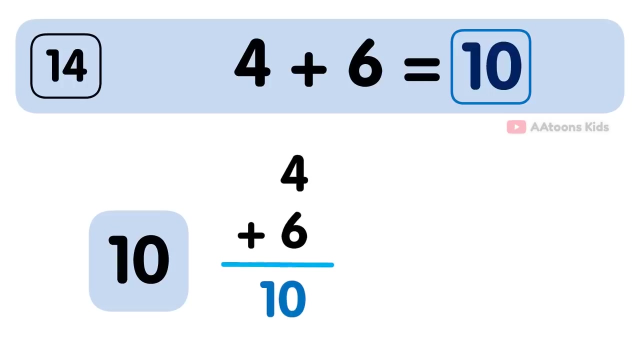 8 plus 7 is equal to 15.. The answer to 8 plus 7 is 15.. 4 plus 6 is equal to 10.. The answer to 4 plus 6 is 10.. 1 plus 3 is equal to. 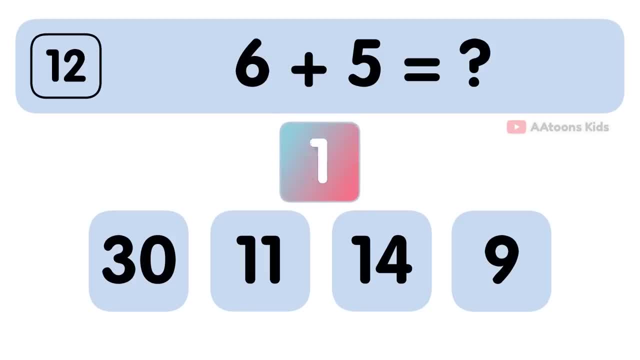 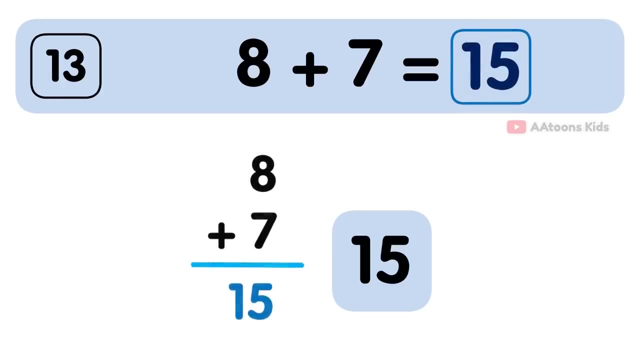 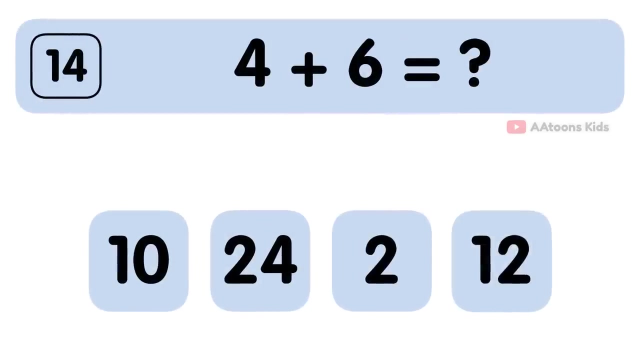 11.. The answer to 6 plus 5 is 11.. 8 plus 7 is equal to 15.. The answer to 8 plus 7 is 15.. 4 plus 6 is equal to 10.. The answer to 4 plus 6 is 10.. 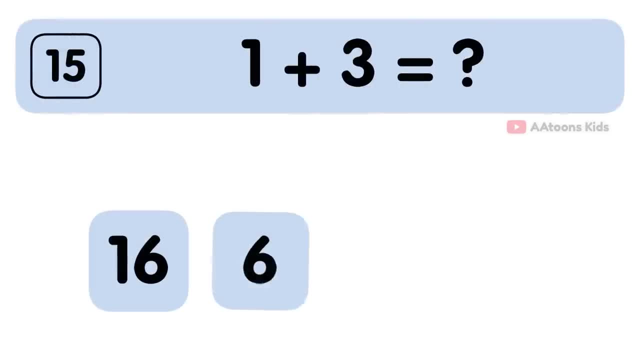 1 plus 3 is equal to 4.. The answer to 1 plus 3 is 4.. 9 plus 2 is equal to 11.. The answer to 9 plus 2 is 11.. 7 plus 6 is equal to. 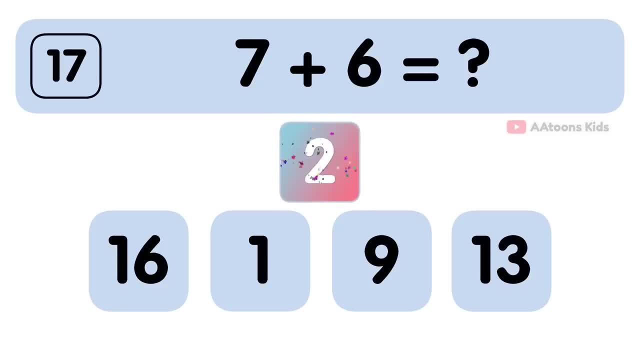 13.. The answer to 7 plus 6 is 13.. 5 plus 8 is equal to 13.. The answer to 5 plus 8 is 13.. 2 plus 5 is equal to 7.. The answer to 2 plus 5 is 7.. 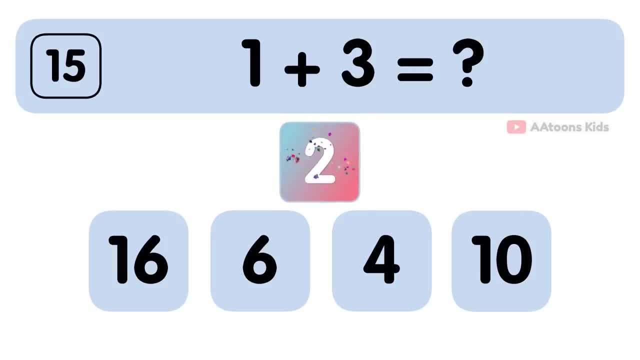 4.. The answer to 1 plus 3 is 4.. 9 plus 2 is equal to 11.. The answer to 9 plus 2 is 11.. 7 plus 6 is equal to 13.. The answer to 7 plus 6 is 13.. 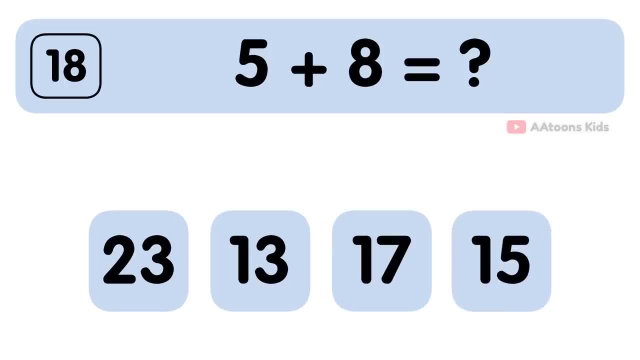 5 plus 8 is equal to 13.. The answer to 5 plus 8 is 13.. 2 plus 5 is equal to 7.. The answer to 2 plus 5 is 7.. 1 plus 7 is equal to. 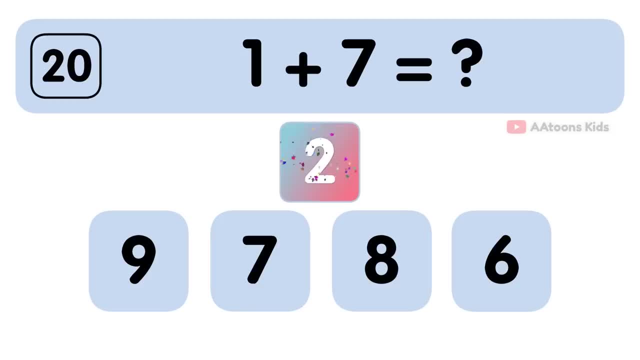 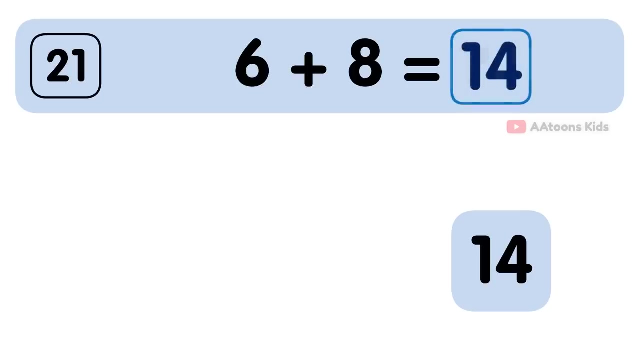 12. 8.. The answer to 1 plus 7 is 8.. 6 plus 8 is equal to 10.. 14. The answer to 6 plus 8 is 14.. 4 plus 7 is equal to 11.. The answer to 4 plus 7 is 11.. 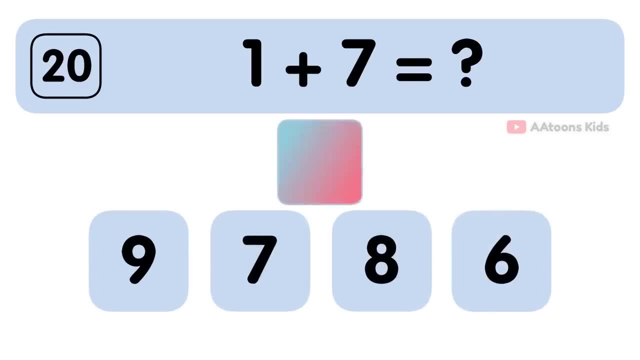 1 plus 7 is equal to 12.. 6 plus 3 is equal to 9. 8. The answer to 1 plus 7 is 8.. 6 plus 8 is equal to 14.. The answer to 6 plus 8 is. 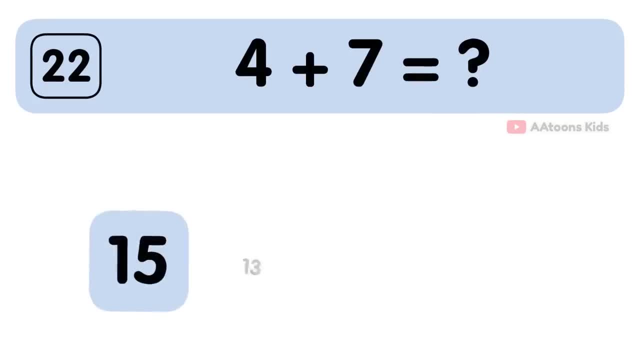 14. 14. 4 plus 7 is equal to 11.. The answer to 4 plus 7 is 11.. 9 plus 4 is equal to 13.. The answer to 9 plus 4 is 13.. 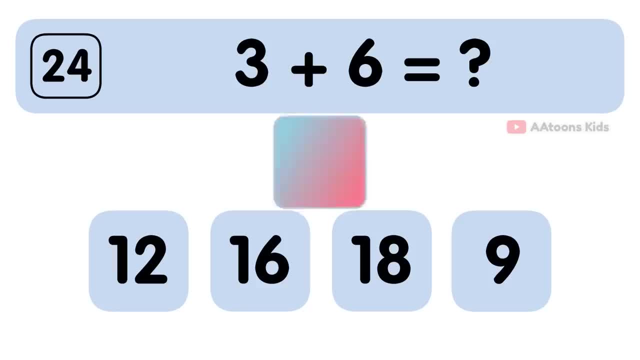 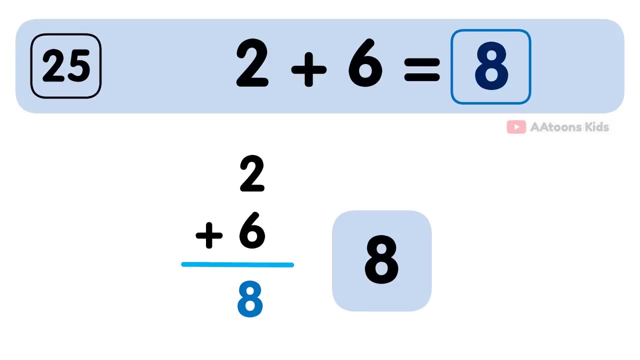 3 plus 6 is equal to 9.. The answer to 3 plus 6 is 9.. 2 plus 6 is equal to 8.. The answer to 2 plus 6 is 8.. 4 plus 2 is equal to. 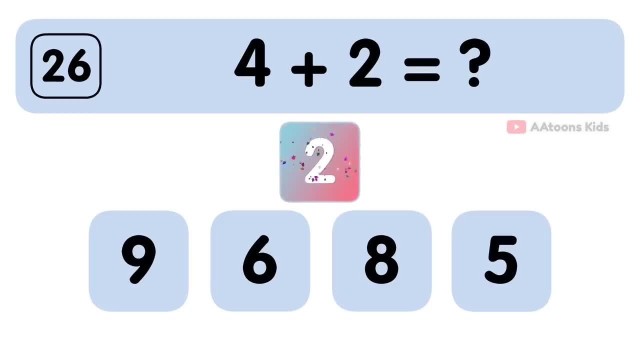 6.. The answer to 4 plus 2 is 6.. 8 plus 3 is equal to 11.. The answer to 8 plus 3 is 11.. 4 plus 4 is equal to 8.. The answer to 8 plus 3 is 8.. 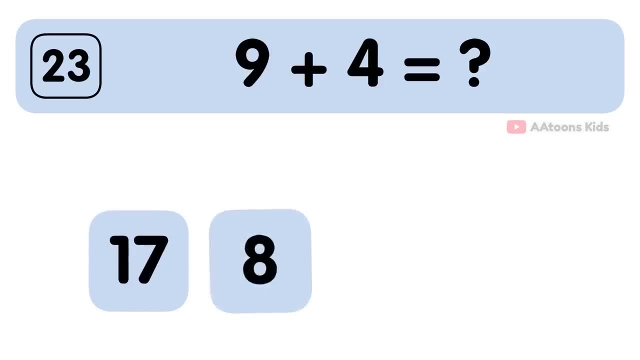 15.. 9 plus 4 is equal to 13.. The answer to 9 plus 4 is 13.. 16.. 3 plus 6 is equal to 3.. The answer to 3 plus 6 is equal to 3.. 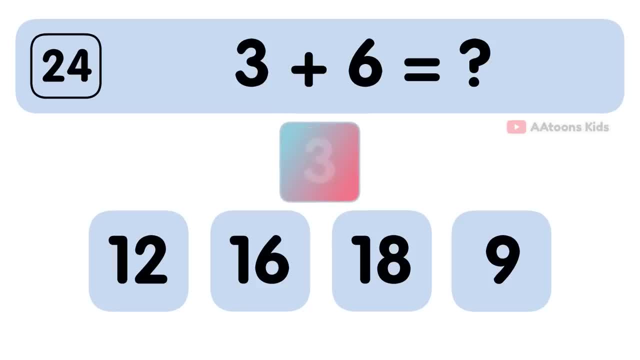 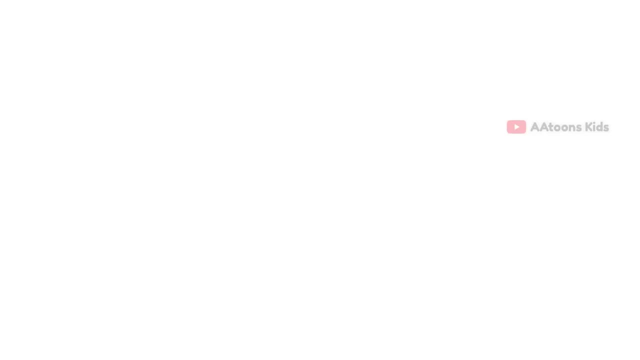 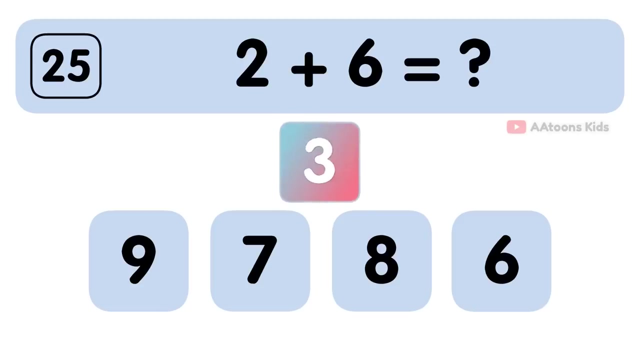 17.. 3 plus 6 is equal to 9.. The answer to 3 plus 6 is 9.. 18.. 2 plus 6 is equal to 9.. The answer to 3 plus 6 is 9.. 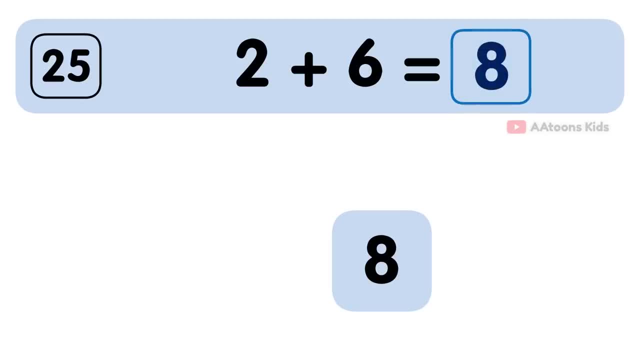 19. 8.. The answer to 2 plus 6 is 8. 20.. 4 plus 2 is equal to 8.. The answer to 4 plus 2 is 8. 21. 6. The answer to 4 plus 2 is 6.. 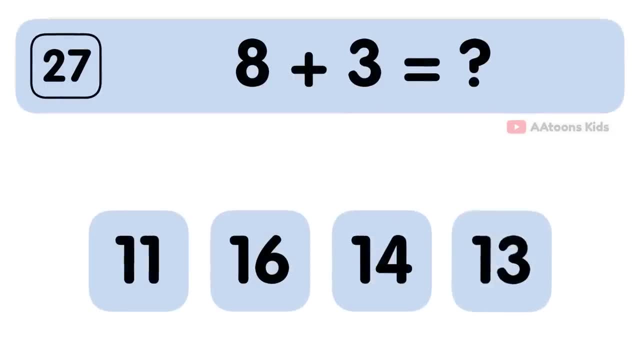 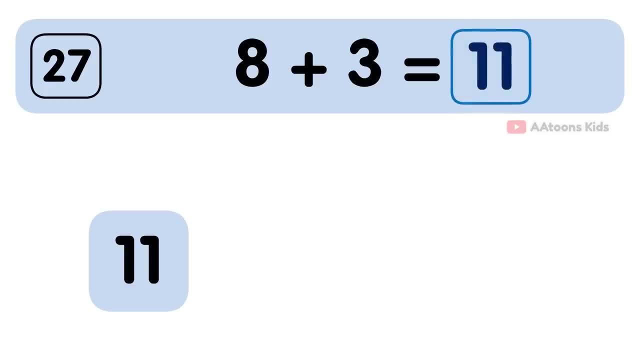 11. The answer to 8 plus 3 is 11.. 4 plus 4 is equal to 8.. The answer to 4 plus 4 is 8.. 7 plus 9 is equal to 16.. The answer to 7 plus 9 is 16.. 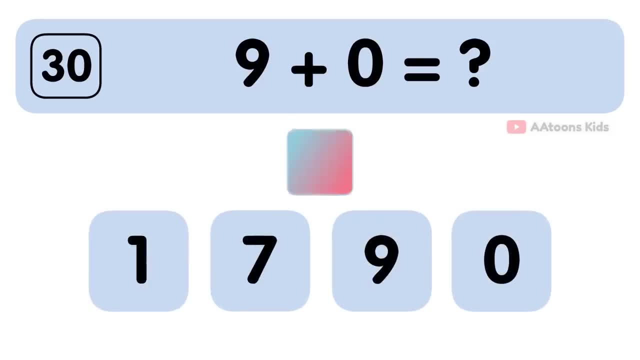 9 plus 0 is equal to 8.. The answer to 9 plus 9 is 8. 9.. The answer to 9 plus 0 is 9.. 6 plus 9 is equal to 15.. The answer to 6 plus 9 is 15.. 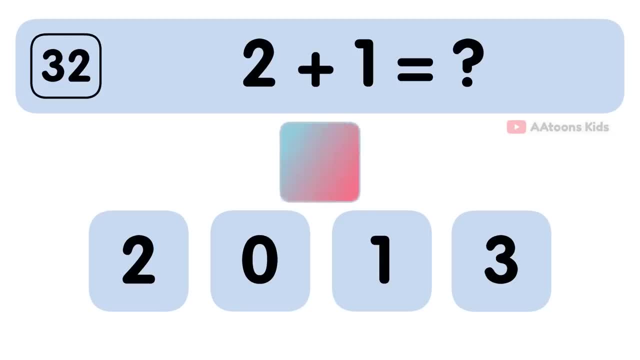 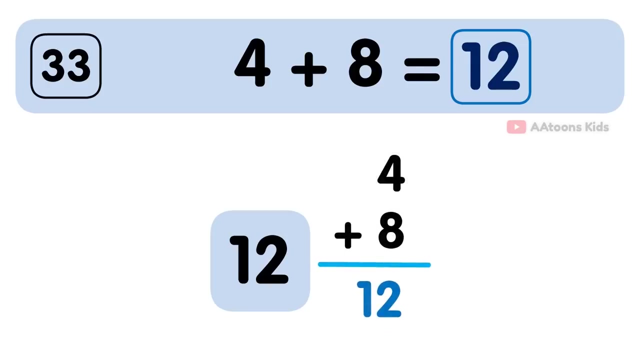 2 plus 1 is equal to 3.. The answer to 2 plus 1 is 3.. 4 plus 8 is equal to 12.. The answer to 4 plus 8 is 12.. 3 plus 9 is equal to. 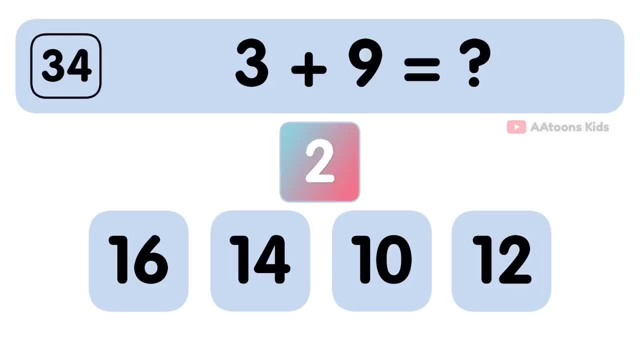 12.. The answer to 3 plus 9 is 12.. 3 plus 9 is equal to 1 plus 5 is equal to 6.. The answer to 4 plus 9 is 12. 6.. The answer to 1 plus 5 is 6.. 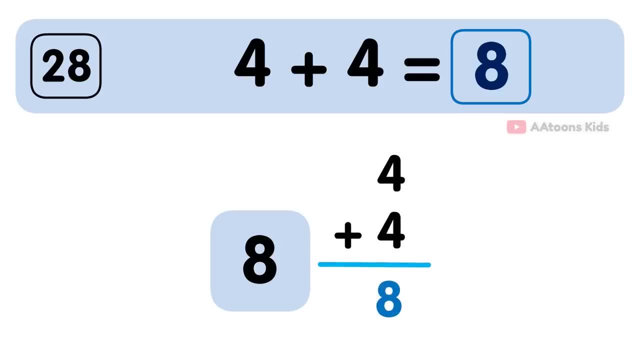 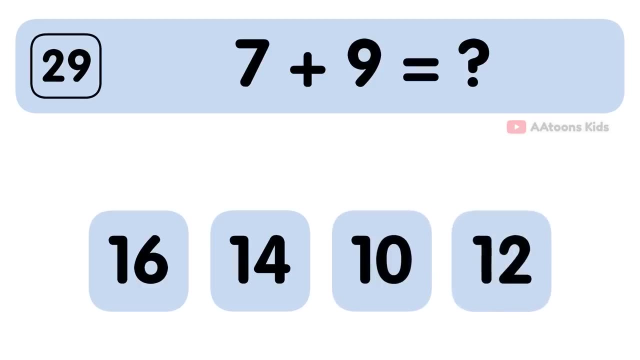 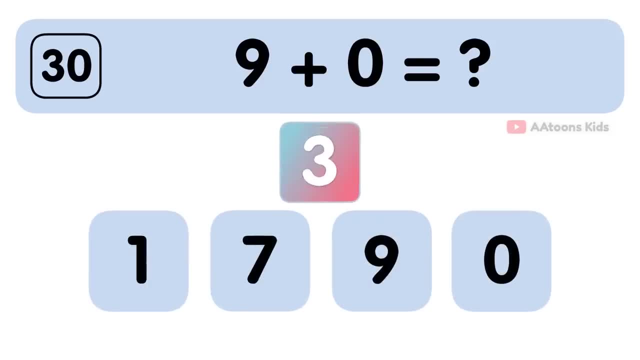 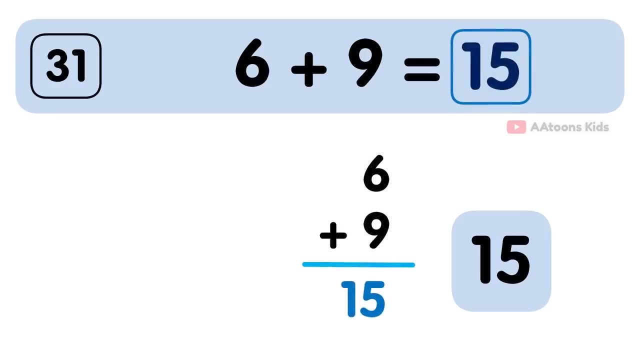 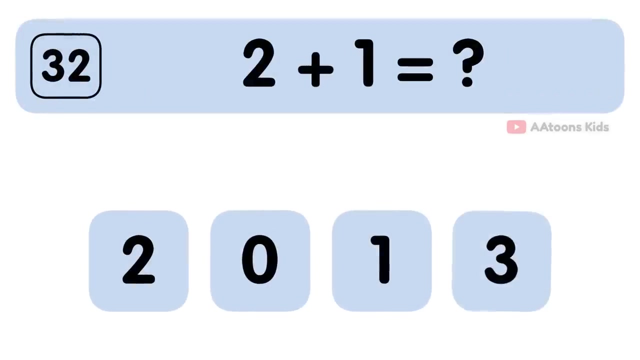 9 plus 0 is equal to 9.. The answer to 9 plus 0 is 9.. 6 plus 9 is equal to 15.. The answer to 6 plus 9 is 15.. 2 plus 1 is equal to. 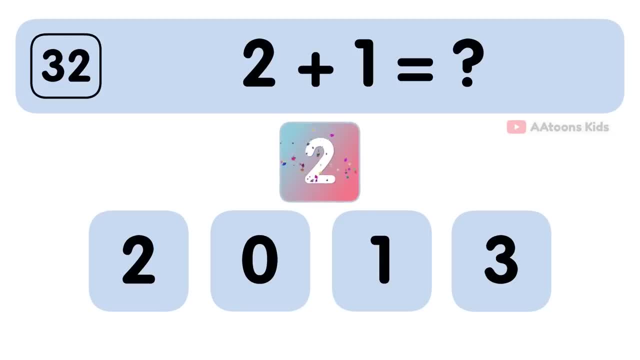 3.. The answer to 2 plus 1 is 2.. 2 plus 1 is equal to 2.. 2 plus 1 is 3.. 4 plus 8 is equal to 12.. The answer to 4 plus 8 is 12.. 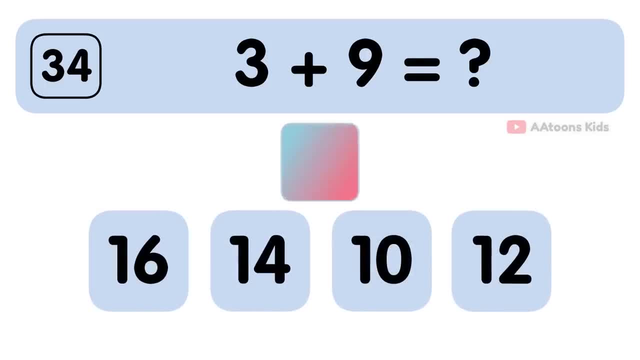 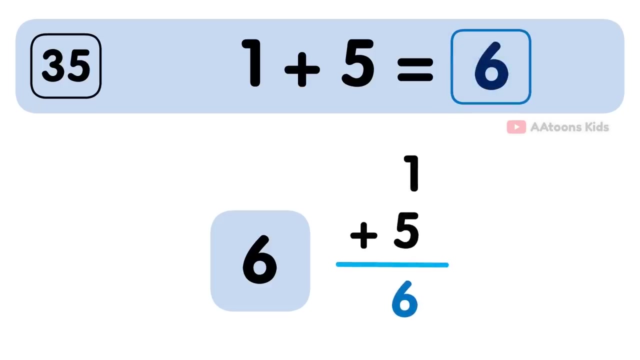 3 plus 9 is equal to 12.. The answer to 3 plus 9 is 12.. 1 plus 5 is equal to 6.. The answer to 1 plus 5 is 6.. 8 plus 4 is equal to. 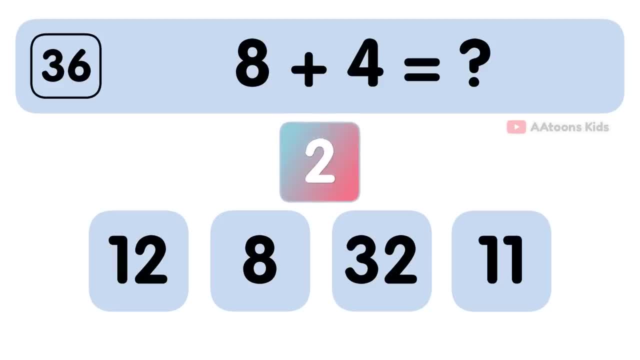 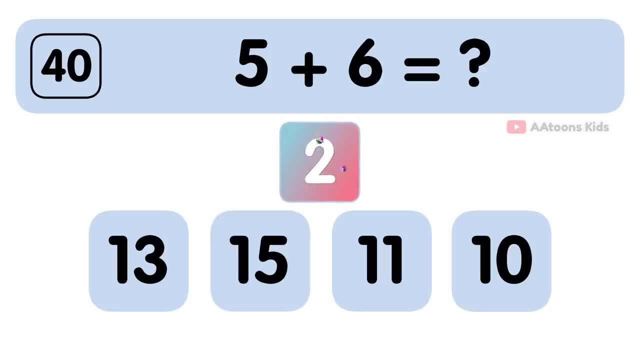 12. The answer to 4 plus 9 is 12.. 11. The answer to 5 plus 6 is 11..